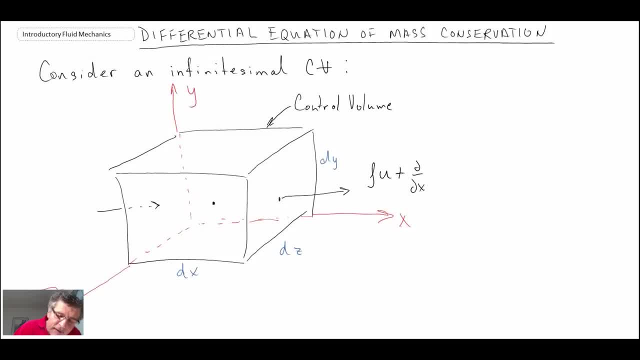 So this is assuming that we're expanding this about the very center of our control volume cube, Okay, Okay, So there we have mass flux. Here's the flux. Let's check out another expression. Let's check out a material coming in on the back surface and mass flux leaving the front surface. and this we are going. 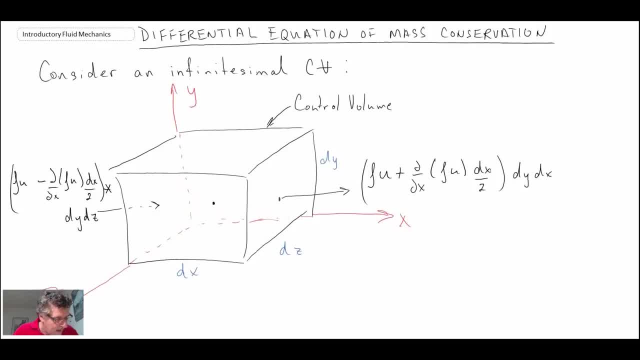 to apply for all three directions. The other thing that we have is we can look at our continuity equation or the conservation of mass for our little differential element here. So I'm going to write that out And we know from all of our control volume analysis that that is zero. 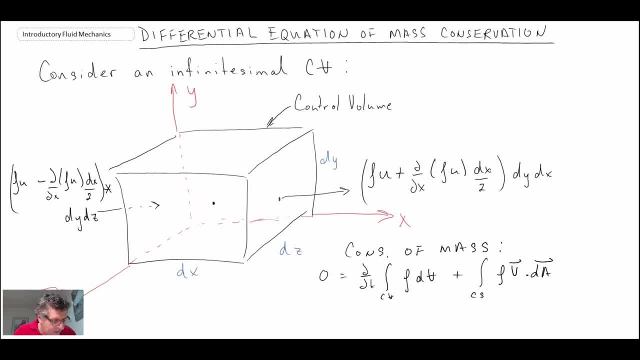 So that is what we did in our control volume analysis. And for the second term here we're going to use the Taylor series expansion- Oops, I should have written that in there. This is a Taylor series expansion and it is used quite often whenever you're deriving differential element equations like you would use here with the finite difference. 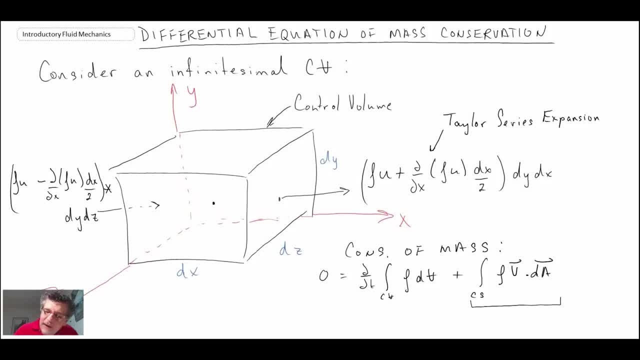 method or a numerical approach. But this term here we're going to look at in a moment. Before we get to that, let's take a look at the first term here, And this first term we can re-express that as being the time rate of change of, and it's going to be just the volume of the 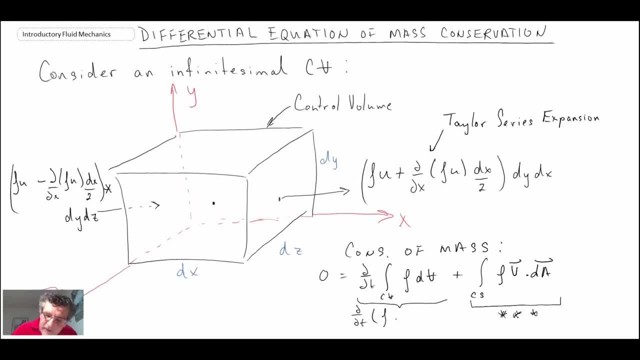 differential element. So it's the density and the volume of the differential element is dx, dy, dz. So we can replace that first term and then for the second term we have to look at mass flux coming into and out of each of the surfaces in our little tiny 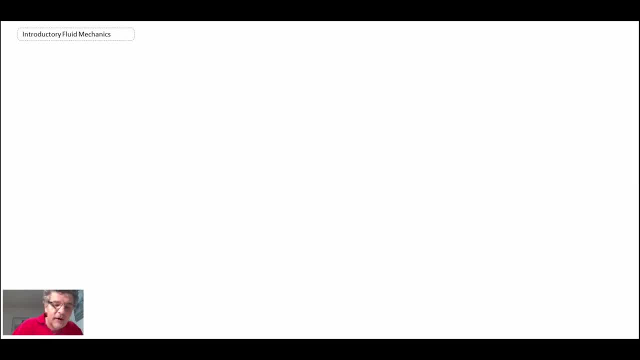 cube. So let's take a look at the second term in our control volume equation And what we had was an integral over the control surfaces of rho, v, dot, da. So I can look at mass flux in the x direction. to begin with, And, just like when we did with control volume analysis, we had to look at the 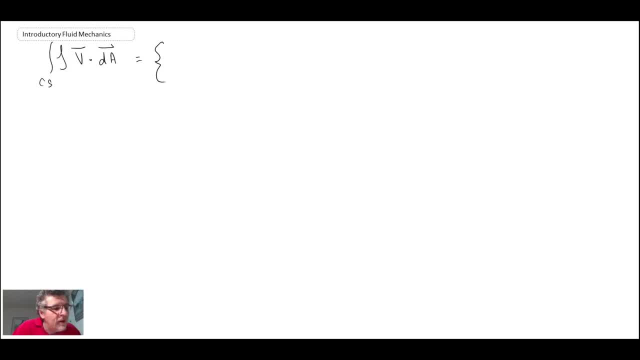 sine of which the flow was coming in. And so the left hand surface is going to have a situation where, if I draw out a sine, we have a velocity coming. The area vector is pointing out in that direction, Velocity in that direction. So the dot product there is going to 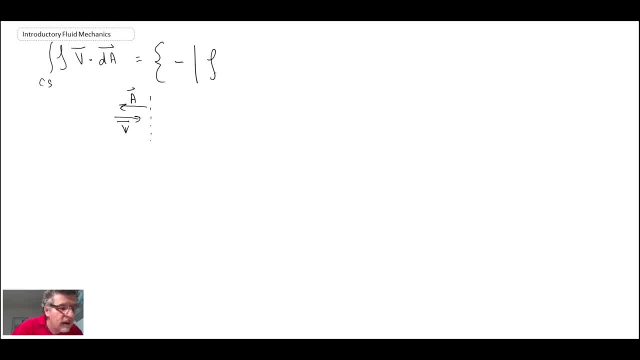 result in a negative value. And then for the right hand surface, the dot product for that one is going to be positive, and when w I'm going to, u are picked up, I'm however I am. and similarly we could do the same for the Y face and then again for the Z or Z face. 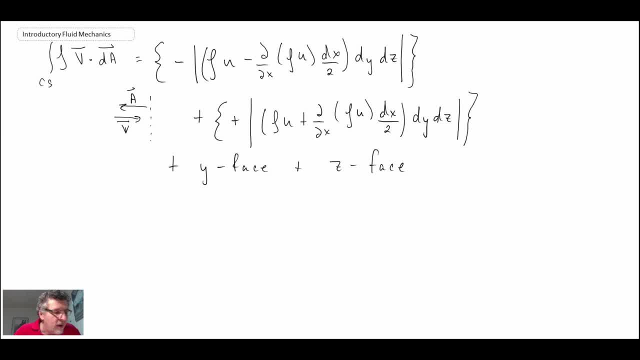 Okay. so when we expand all of this and do it for the X, the Y, the Z face, and then we bring in the time rate of change of the mass of the control volume, our continuity equation for our little element starts to look something like this: 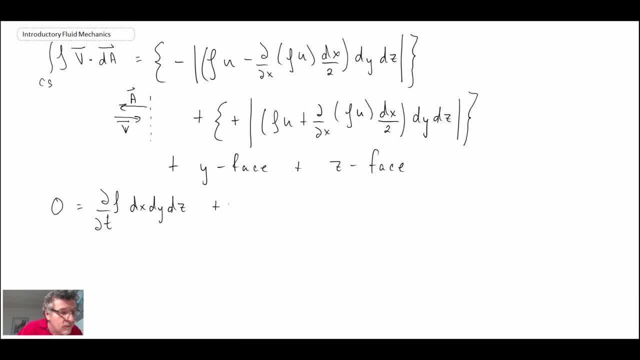 And that can be rearranged to the following: And what we're going to do here: the volume's going to cancel out. Okay, so we get to this point. Now, what can we do with this equation here? Well, the partial rho, partial T, that's fine, but it's this one that we're going to take a look at. 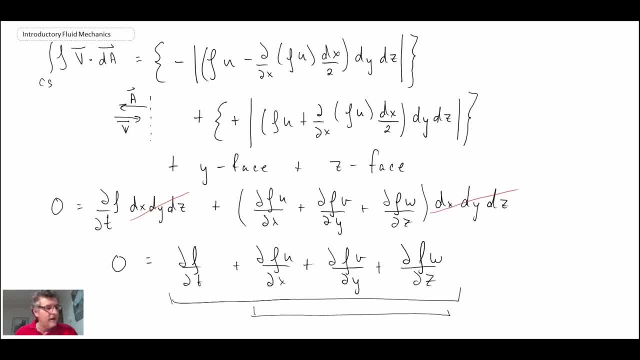 And we're going to look at some of the vector operators that we've covered thus far, And the way we're going to do that is we're going to take a look at the vector operators that we've covered thus far, And the ones we're going to look at is going to be the gradient and divergence operators. 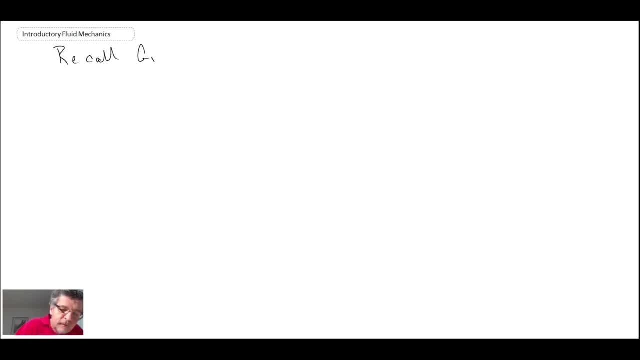 So, if you recall gradient- and gradient was defined as being and divergence- what we had was del dot, some vector, So I'm going to apply it to an arbitrary vector A And remember the divergence, or del dot operator takes a vector and converts it into a scalar. 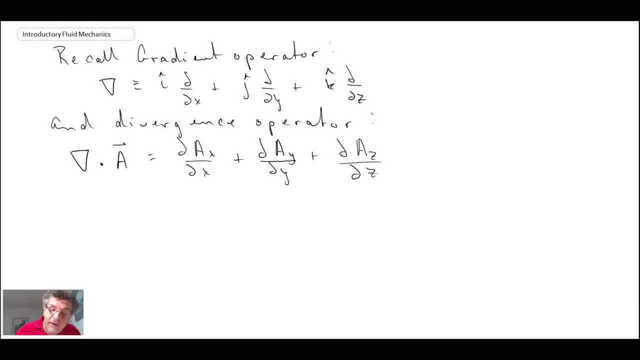 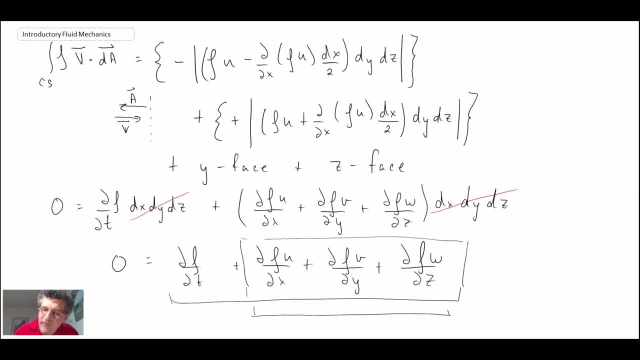 So what we have, we can use these two operators. Okay, Looking back at our equation, we're going to use the divergence operator to recast that, So let's go ahead and do that, And what we end up with is something that looks like the following: 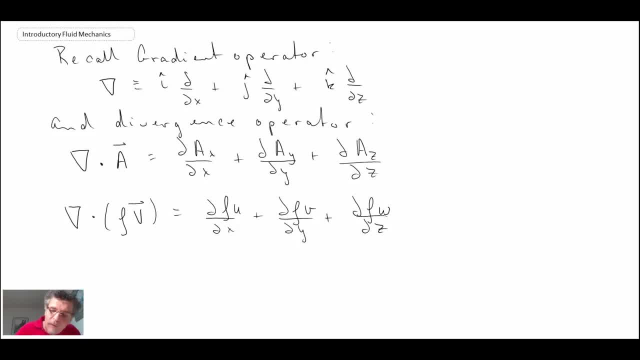 So if we look back at our equation, we can see the divergence of rho times. the vector v is exactly what we have for the second part of our equation And consequently we can rewrite continuity to look something like this: So that is an important equation.